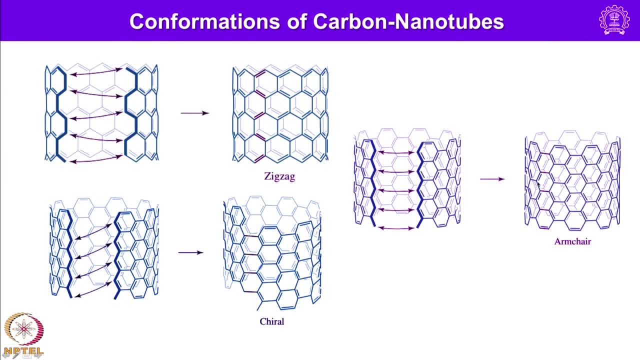 center. or one can also make in this way: This gives a chiral center. or one can also make in this way: This gives a chiral center. or one can also make like this armchair, something like this. So there are several ways in which the clipping of the edges 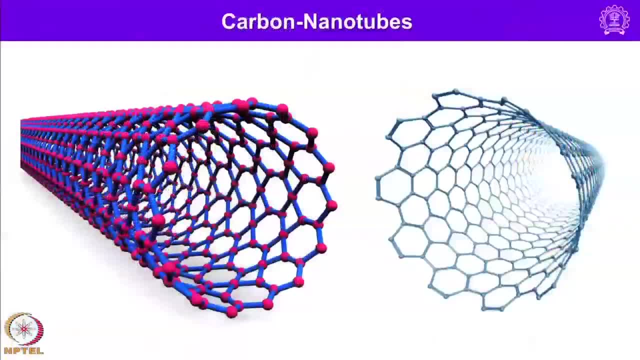 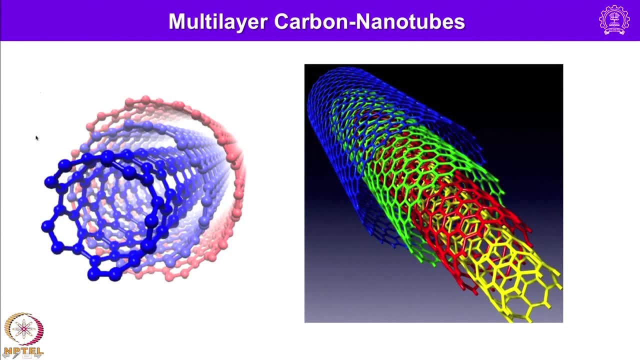 can be performed. ok, So this is how a typical carbon nanotube looks like. ok, And if I could take a smaller nanotube, put it inside. You can see this one. One can play around. these are called multilayer carbon nanotubes. ok, So let us look into another. 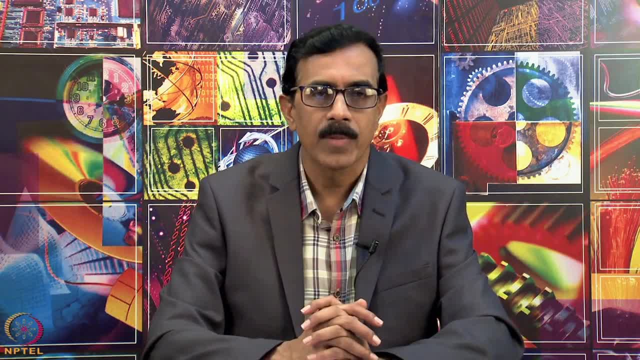 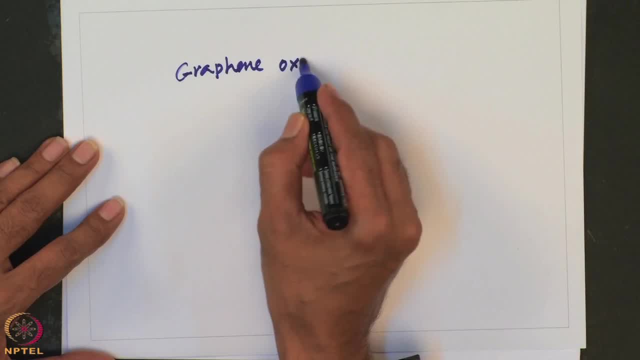 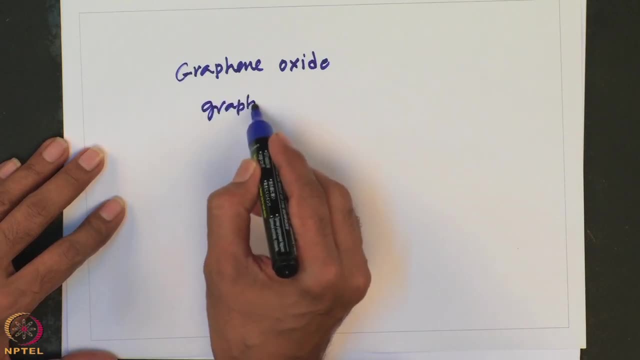 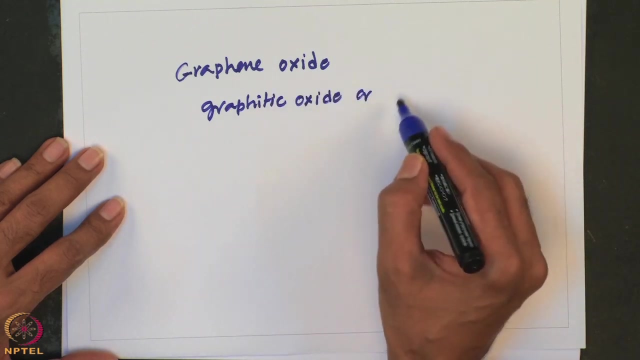 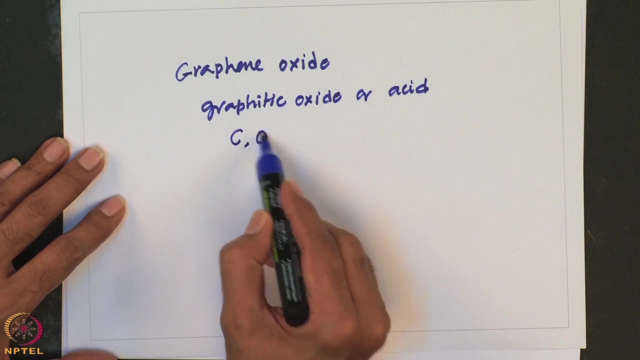 important compound of graphene, that is, graphene oxide. Graphene oxide, formerly called graphitic oxide oxide, is also called graph graphitic oxide or graphitic acid or acid ok, is a compound of carbon, essentially carbon oxygen and hydrogen, in variable ratios by the oxidation of graphite. 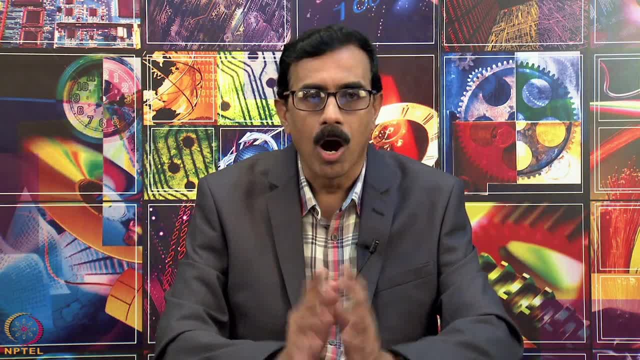 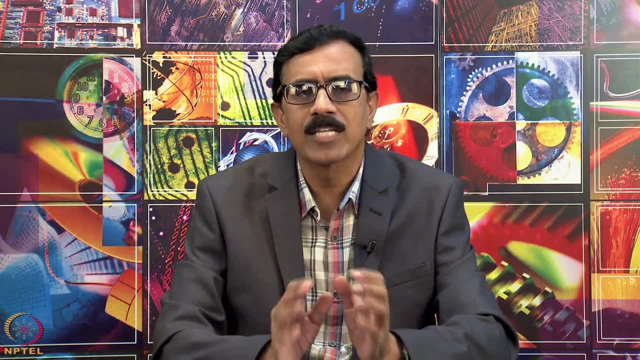 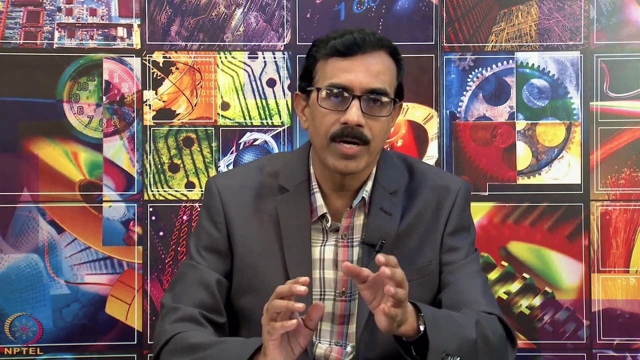 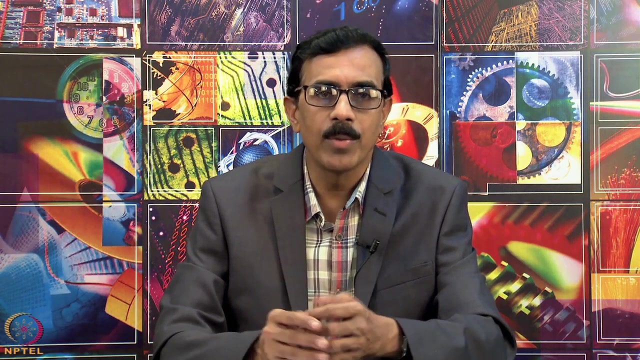 or graphene. using strong oxidizing agents, oxygenated functionalities are introduced in the graphite structure, which not only expand the layer separation but also makes the material hydrophilic. You should remember, graphene or graphite is hydrophobic, but adding this oxygenated functionalities one can make the material hydrophilic. Graphite oxide is 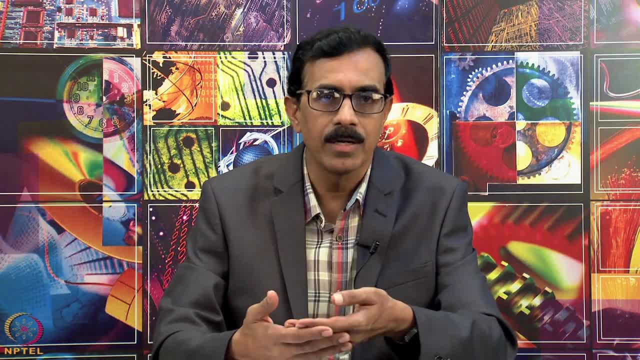 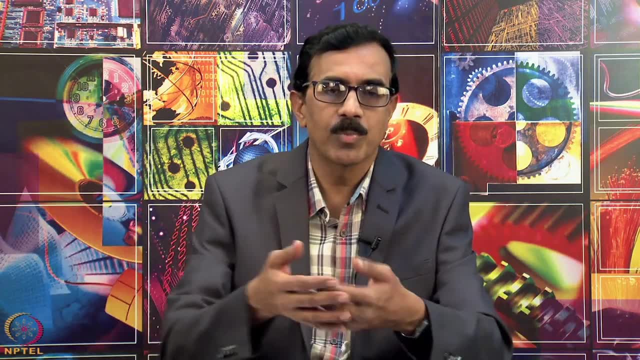 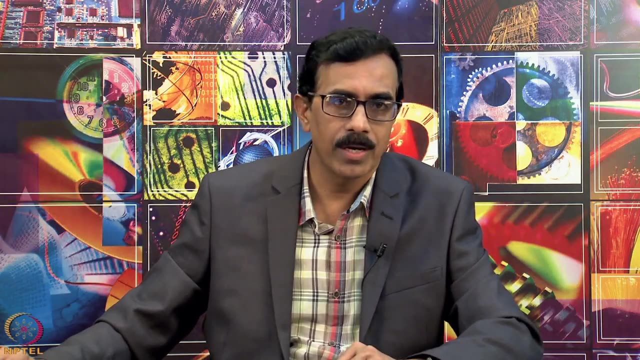 a multilayer system, whereas in a graphene oxide dispersion of few layers or monolayers flakes can be found. That means, dispersion of few layers or monolayer flakes can be found. ok, something like this. ok, Of course one can also put epoxide here or hydroxyl groups. 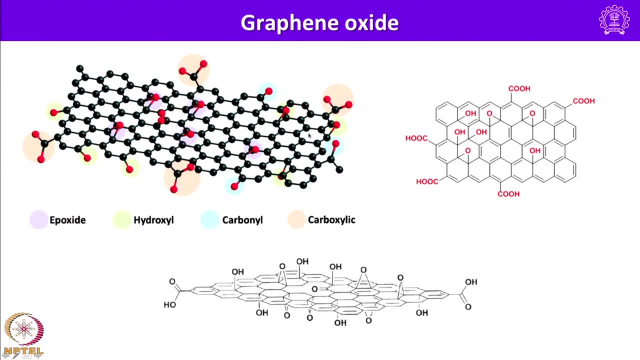 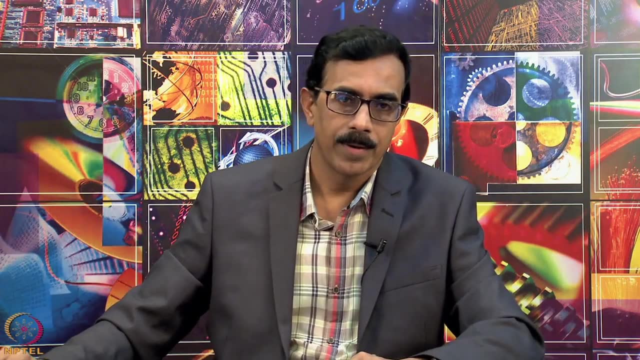 can be added, Or carbonyl groups can be added, or even carboxylic groups can be added, and you can see here and now this is how the dispersion of these groups can be visualized on a single graphene sheet. You can have all kind of oxygenated functionalities. ok, on the surface of graphene. ok, Let us look. 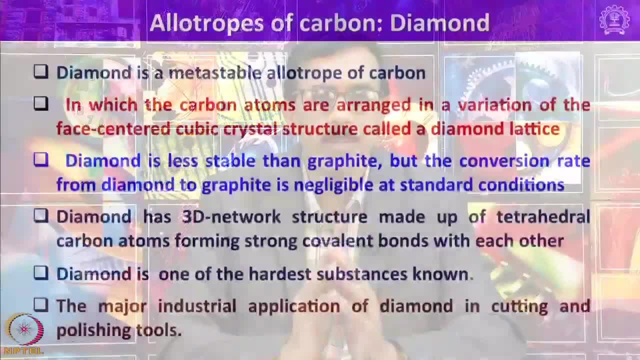 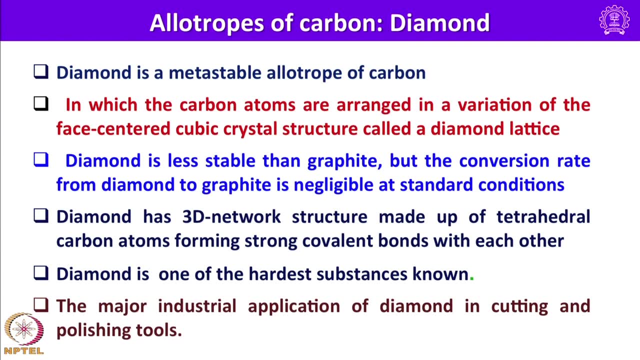 into other allotrope of carbon, that is, diamond. Diamond is a metastable allotrope of carbon in which The carbon atoms are arranged in a variation of the phase centered cubic crystal structure called a diamond lattice. In fact, in carbon, what happens? every carbon atom is tetrahedral. 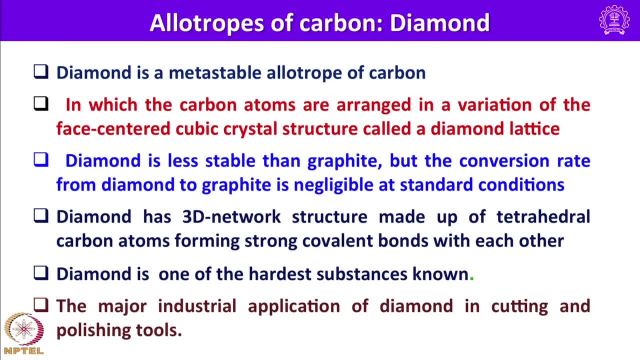 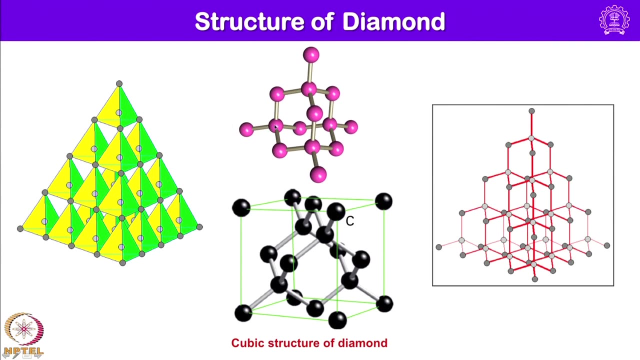 and coordinated to another carbon atom, and this network is three dimensional in nature. that leads to the formation of diamond. ok, So diamond is one of the hardest substance known. The major industrial application of diamond is in cutting and polishing. Ok, And this is how the diamond looks like. So every carbon atom is binding in a tetrahedral. 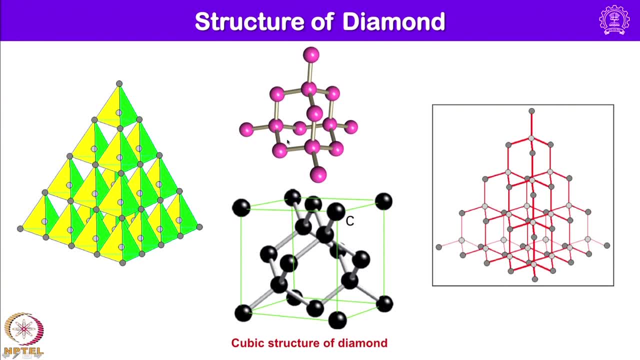 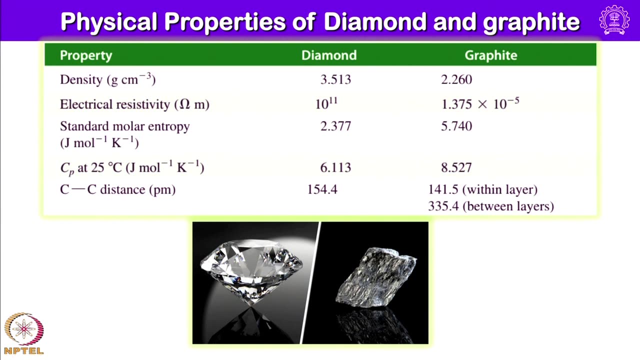 fashion to neighboring carbon atom and this network grows in three dimension. to give this kind of structure here. ok, Cubic structure of diamond can be seen here in this diagram. ok, So let us look into the difference between graphite and diamond density. It is: 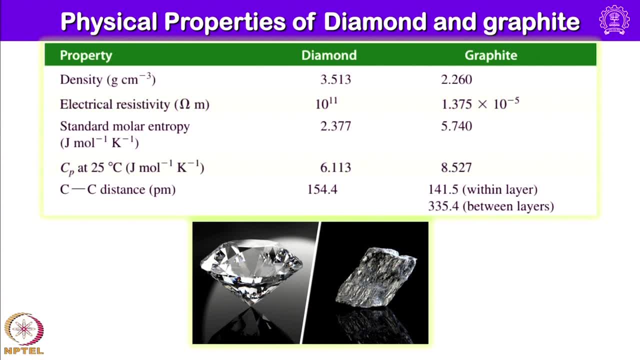 It is. It is more in case of diamond it is 3.513, whereas graphite 2.26. and electrical resistivity is remarkable in case of diamond, 10 to the power of 11, whereas in case of graphite. you can see that. and standard molar entropy is 2.377 in case of diamond, whereas in case of 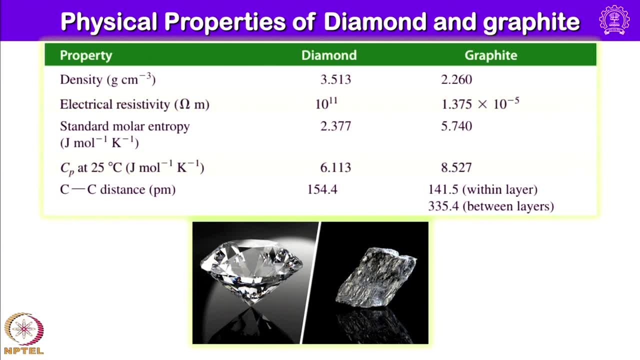 graphite it is 5.740 joules per mole per kelvin, Ok, And carbon-carbon distance is much longer. in case of diamond it is 154 picometer, whereas in case of graphite it is 141.5. within the layer and between the layer, the separation. 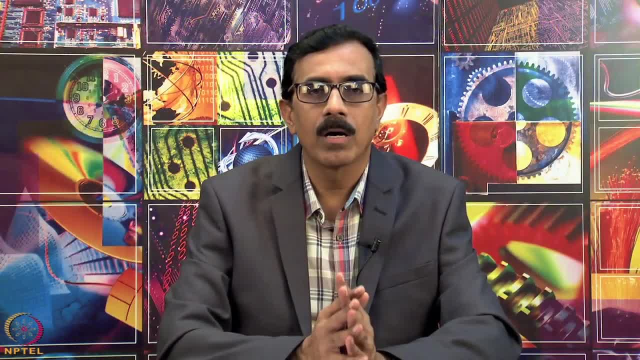 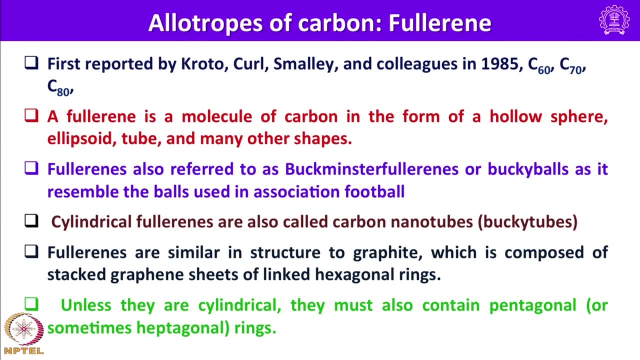 is 335 picometer. Another important allotrope of carbon is fullerene. It was first reported by a three scientists- Crotto, Curl and Kuhn Ok- In 1985 and they showed the presence of C60, C70 as well as C80.. A fullerene is a molecule. 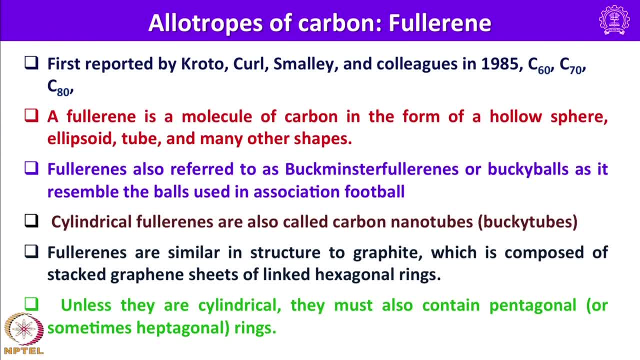 of carbon in the form of a hollow sphere resembling a football- ok. or it can be in the form of an ellipsoid or a tube and can take many other shapes. Fullerenes also referred as Buckminster fullerenes or buckyballs, Ok. 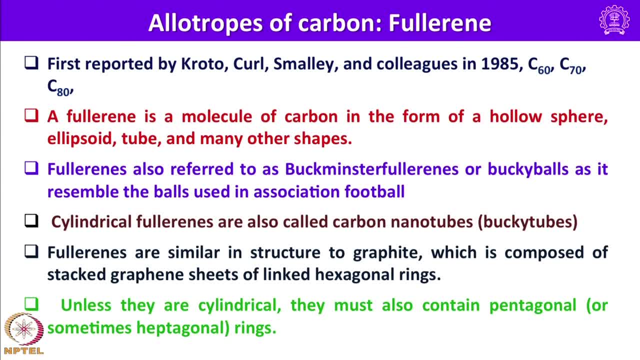 As it resembles the ball used in association football. Cylindrical fullerenes are also called carbon nanotubes- bucky tubes. Fullerenes are similar in structure to graphite, which is composed of stacked graphite sheets of linked hexagonal rings, Unless they are cylindrical. 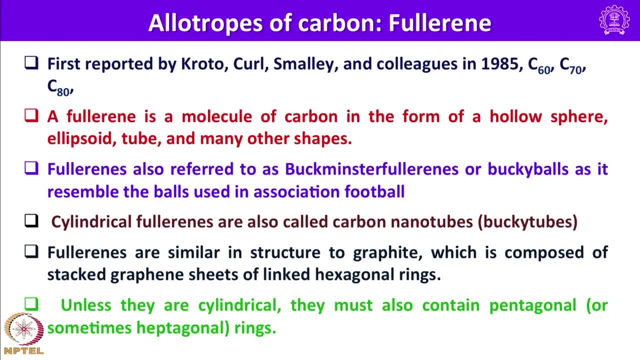 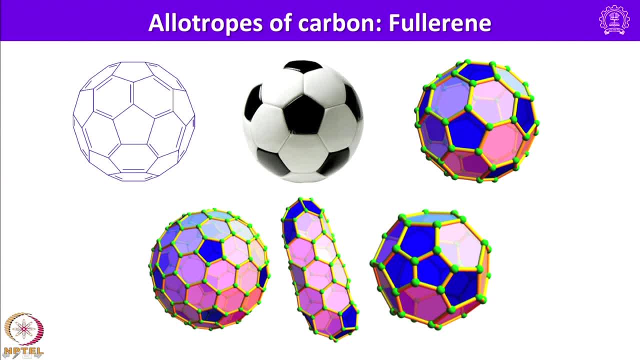 they must also contain pentagonal or sometime, heptagonal rings as well. You can see here fullerene. Ok, It is made up of hexagonal as well as pentagonal rings. and also, you can see here, it is made up of 6 membered as well as 5 membered rings. 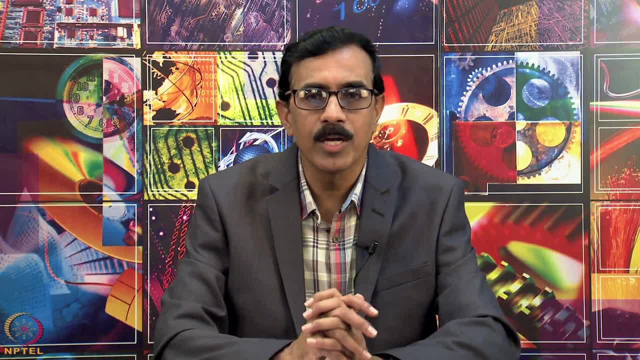 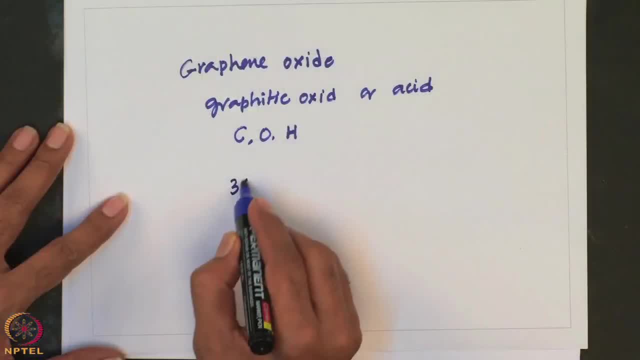 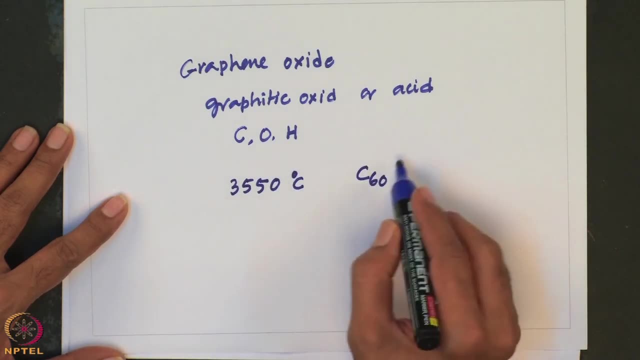 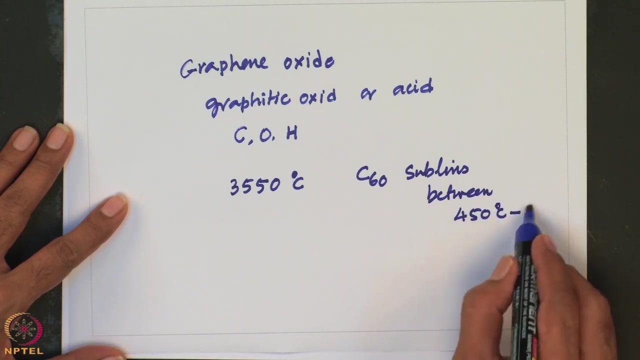 So just let us look into one point here. The melting point of diamond and graphite are greater than 3550 degree centigrade, But carbon 60, ok, C60.. Ok, Ok. So these are the sublimes between 450 degree centigrade to 500 degree centigrade. Why is? 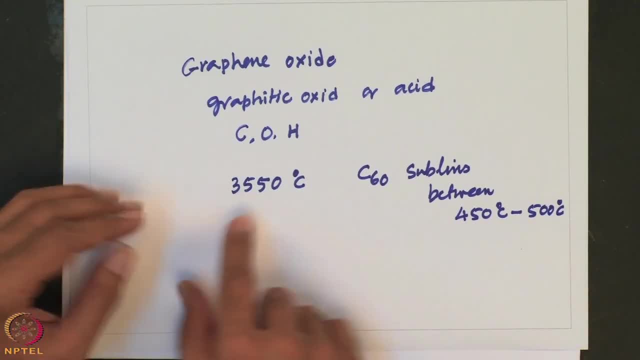 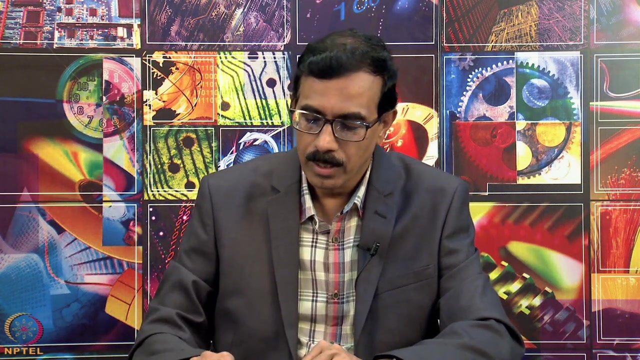 this difference. Ok, Melting point of diamond or graphite is greater than 3550 degree centigrade. Only carbon carbon atoms are there In C60, also only carbon carbon atoms are there, Though hydrogen carbon atoms are there In C80- the hydrogen atom or anything else, But here it sublimes at between 450 to 500. 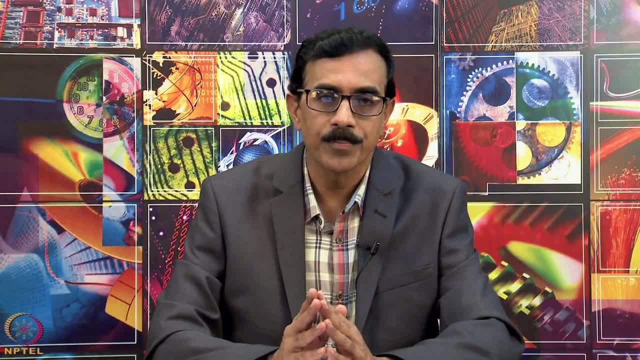 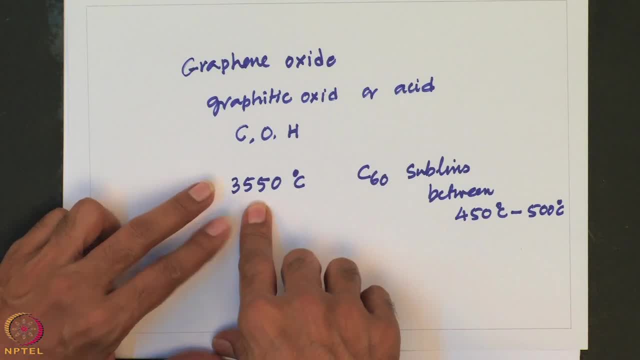 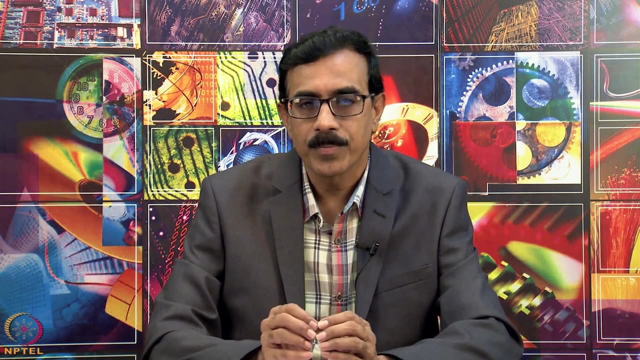 degree centigrade. So that means here one should remember what is the meaning of melting point. and in case of graphite or diamond, melting point means the cleavage of all the bonds associated with diamond. Ok, So that means we have to strip off all the carbon and you have to take individual carbon. 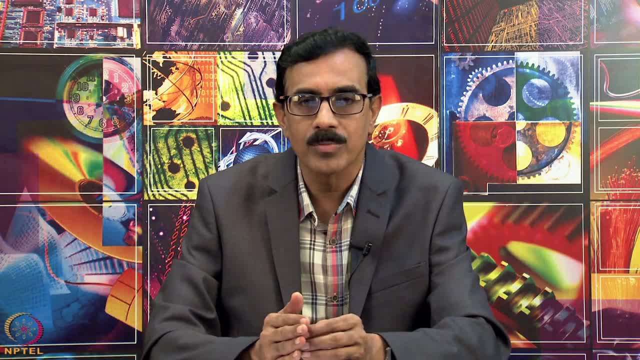 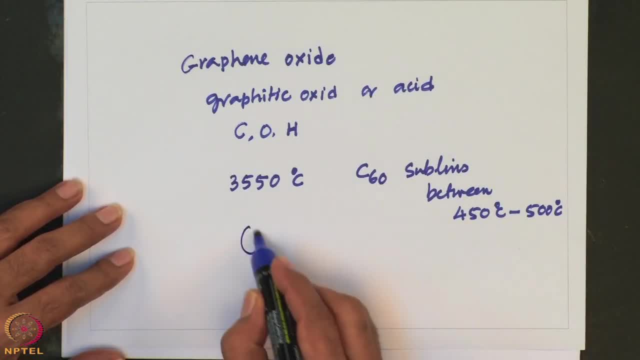 atoms achieve the separation of each carbon atoms, it indicates we achieved melting point, Whereas in case of C 60, C 60 is a molecule, something like this, and in solid state they are arranged in this fashion through some weak interactions In melting point. what happens essentially? 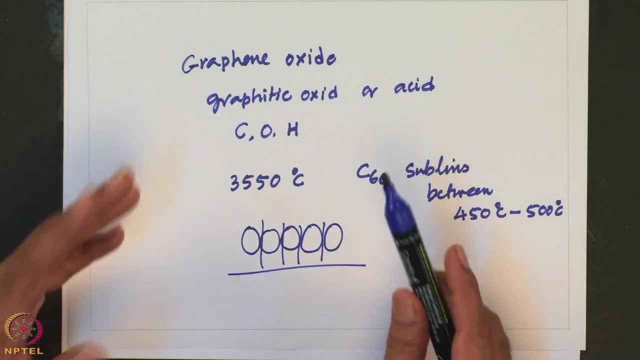 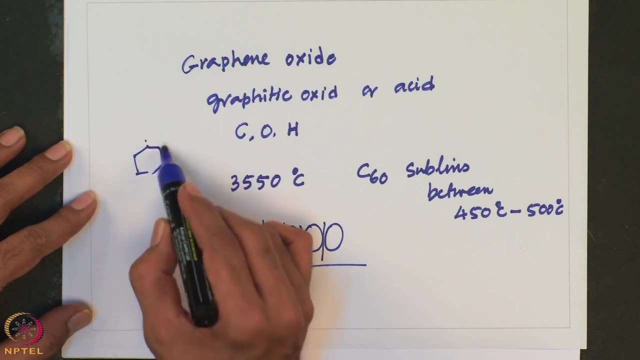 we are separating them, So they are held by weak interactions. as a result, it sublimes at 450 degree centigrade, whereas in case of graphite, if you have something like this, ok, if it continues, the every bond has to be broken, and same thing is to in case of. 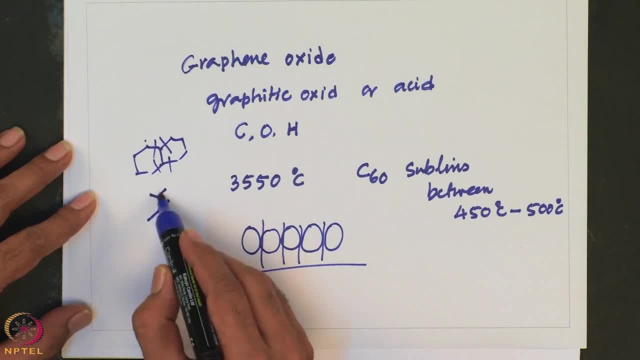 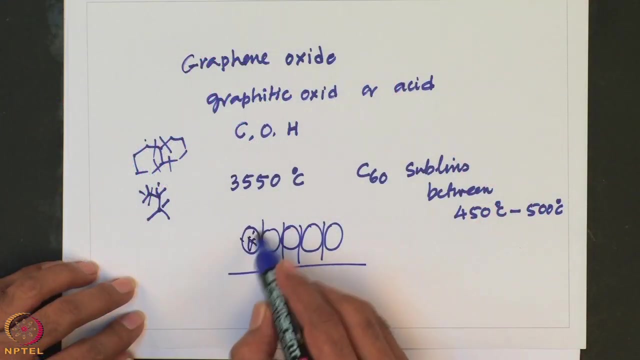 a tetrahedral carbon atom. ok. So here, essentially, we have to cleave all, we have to strip off all carbon atoms from each other to achieve its melting. Same thing is to in case of fullerene. essentially we have to take out this because this itself is a molecule. ok, So this is. 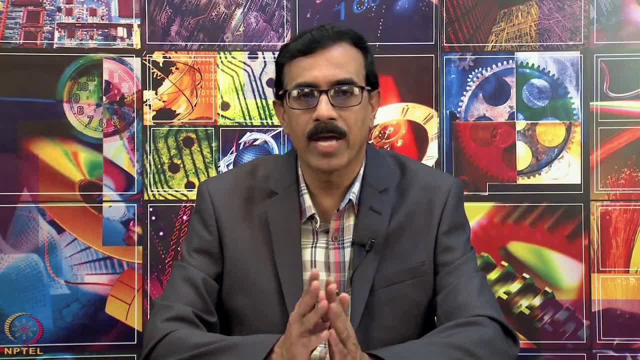 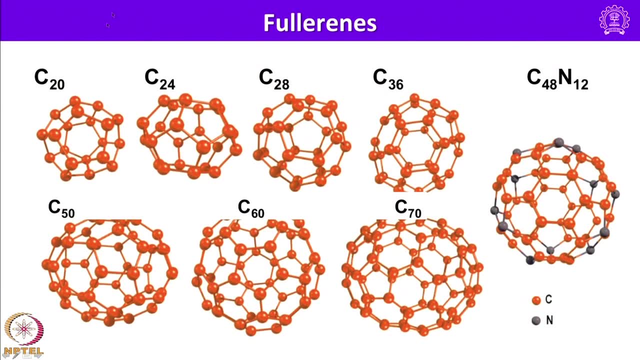 the difference between And the melting point in case of diamond graphite and fullerene. ok, So I have shown you some fullerenes: C 20 and C 24,, C 28,, C 36 and also here this essentially fullerene. 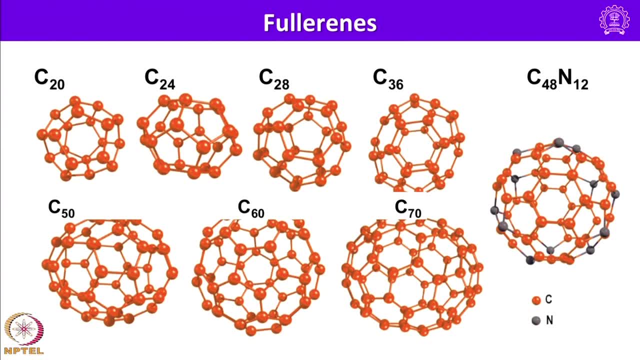 in which 12 carbon atoms are replaced by 12 nitrogen atoms. This is a C 48 and 12, it is a hetero fullerene, and C 50,, C 60 and C 70.. These are some of the important fullerenes. 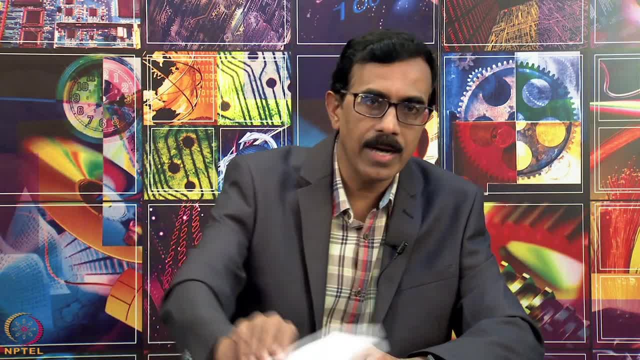 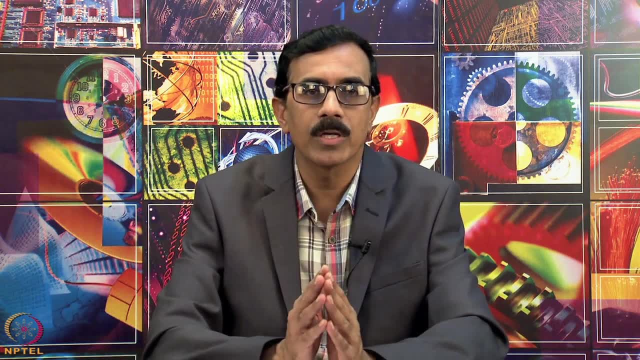 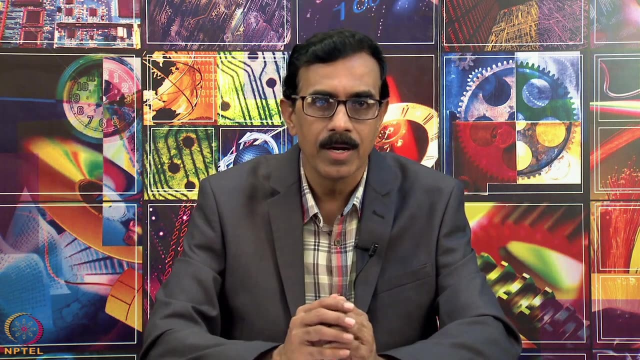 ok, Now let us look into the reactivity of fullerenes. Fullerenes are formed when an electric arc is discharged between carbon electrodes in an inert atmosphere. Although C 60 exhibits a small degree of aromatic character, its reaction tend to reflect the presence of localized double and single bonds, For example. if that is the case, if any olefin having a double-bond undergoes addition reaction, you can anticipate similar addition reactions in case of fullerenes also. In fact it undergoes addition reactions. The ene like nature of C 60 is reflected in. the range of reactions, such as the addition of an oxygen atom to give an epoxide, or addition of ozone at 257 Kelvin to yield an intermediate ozonide like C 60 O 3 or reaction of C 60 with free radicals also can readily occur. 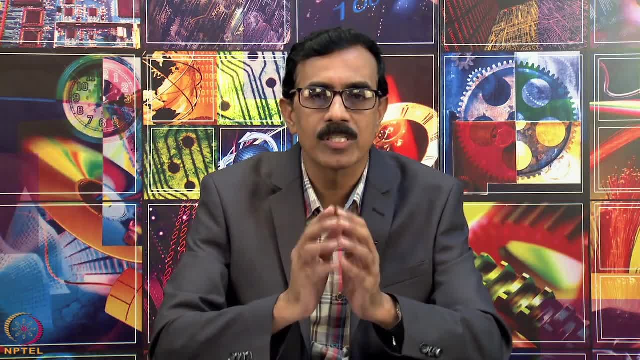 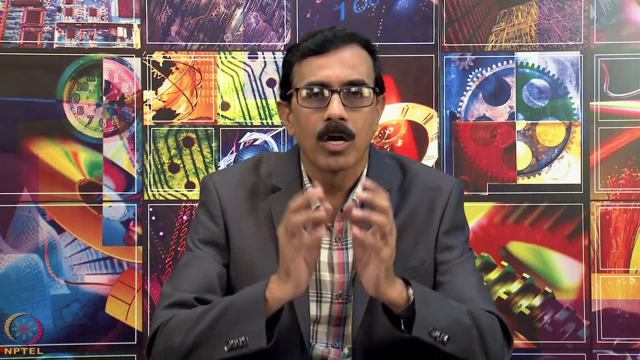 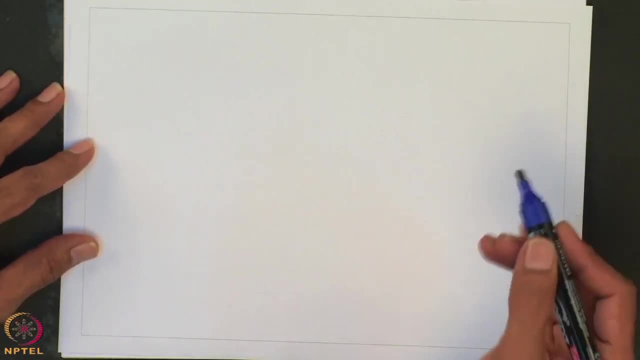 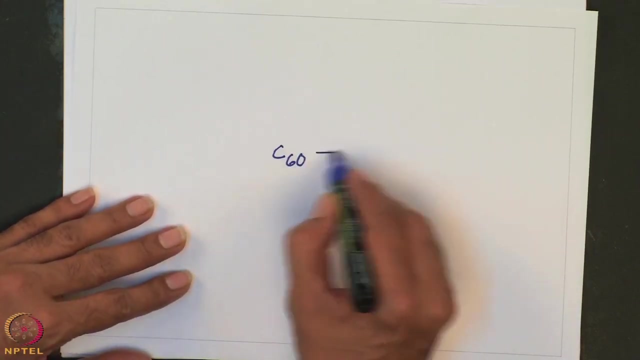 polyhedral fullerenes undergo reversible multi-electron reduction and form complexes with d-block organometallic compounds and also with osmium tetroxide. Let me show you some of these reactions here. Let me write some reactions of C 60.. For example, 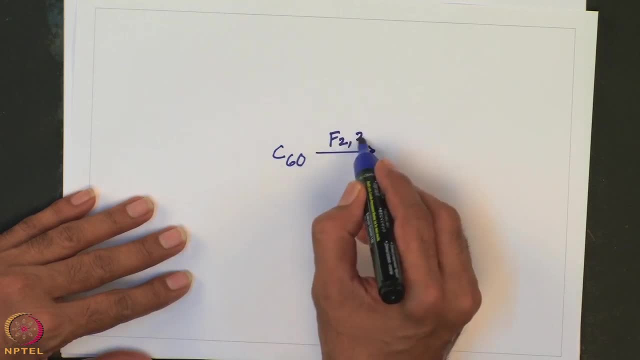 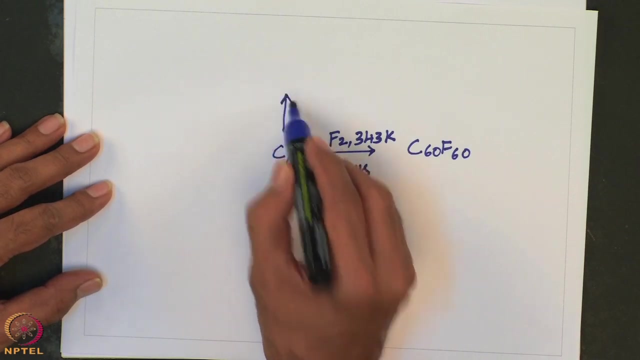 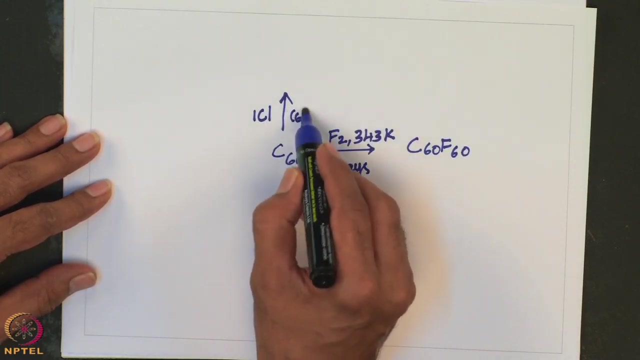 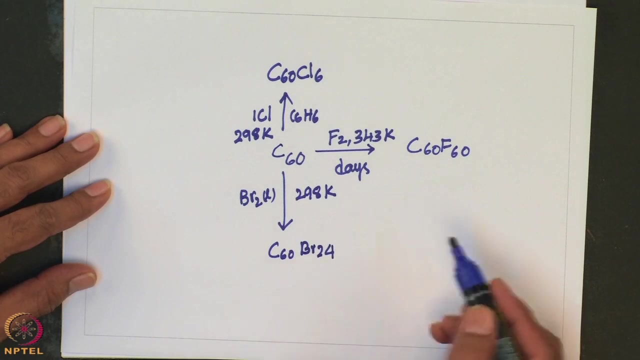 if it is treated with F 2 at 343 Kelvin for days, it forms C 60, F 60.. Similarly, ICl is added in benzene at 298 Kelvin, Ok, it forms C60Cl6. and if you treat with bromine liquid at 298 K, it forms C60Br24, or with 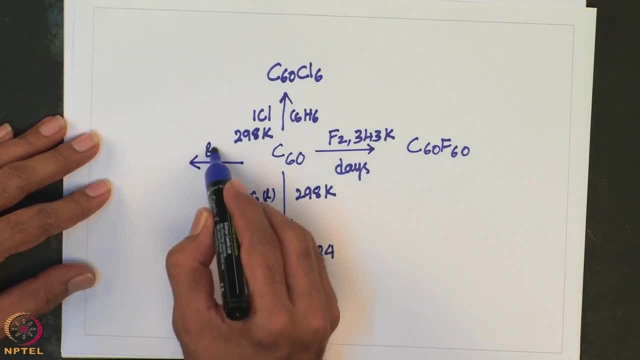 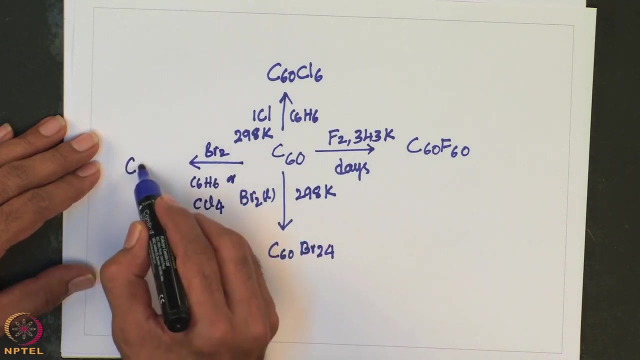 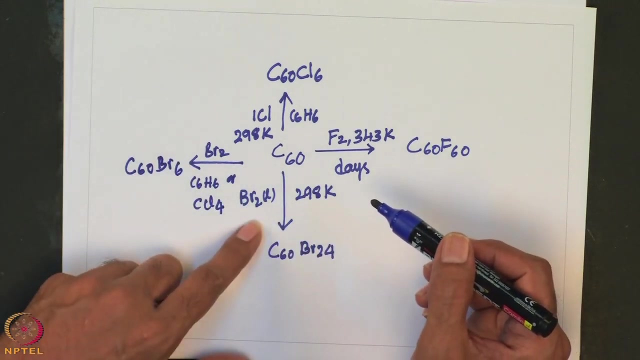 controlled addition of Br2 at 298 Kelvin, only in benzene or carbon tetrachloride, it can give you C60Br6.. So that means, by controlling the amount of bromine we are using, we can either make C60Br24 or one can make C60Br24.. 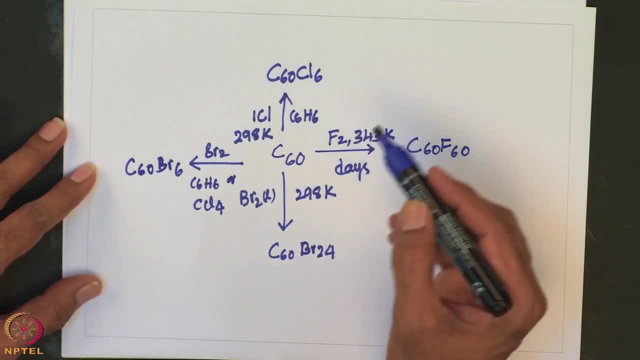 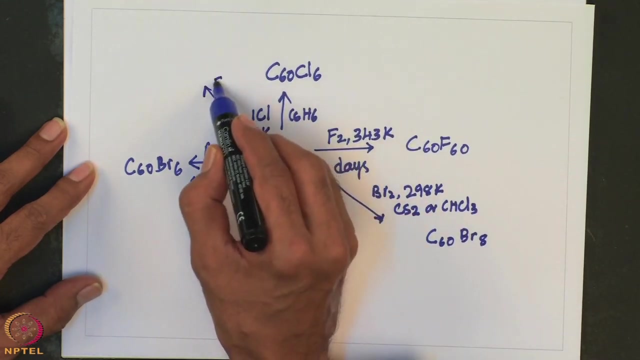 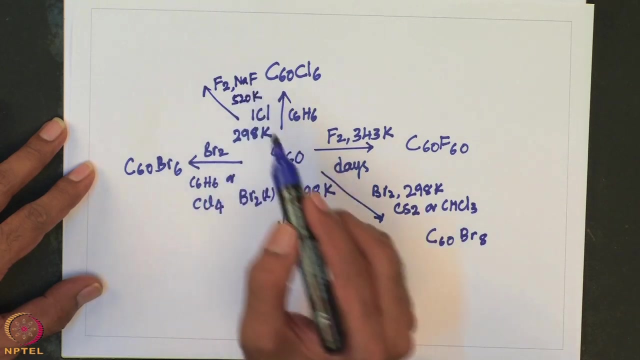 So one can make C60B6.. Similarly one can also use Br2 at 298 Kelvin in carbon disulphide or CHCl3 chloroform to get C60Br8.. You can also take fluorine with the sodium fluoride at 520 Kelvin or directly F2 at 550. 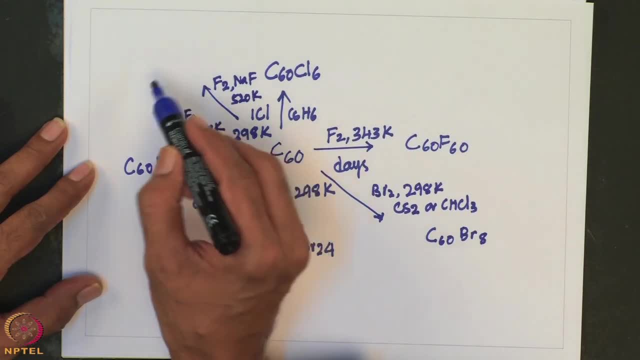 Kelvin. One can get C60F46.. This is the major product. Along with this one, one can add C60Br4.. 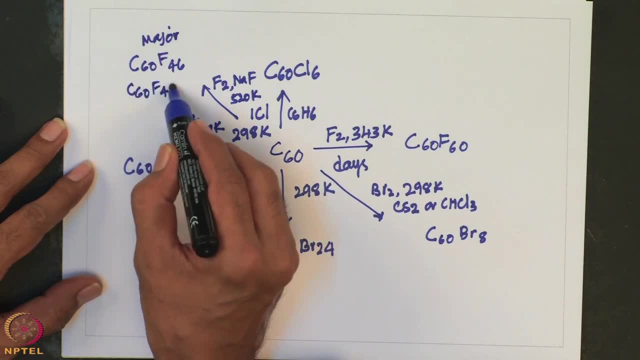 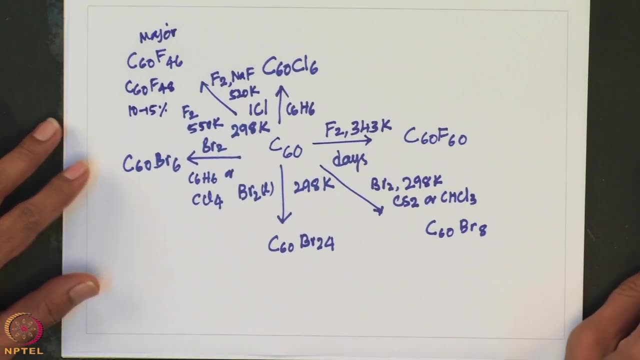 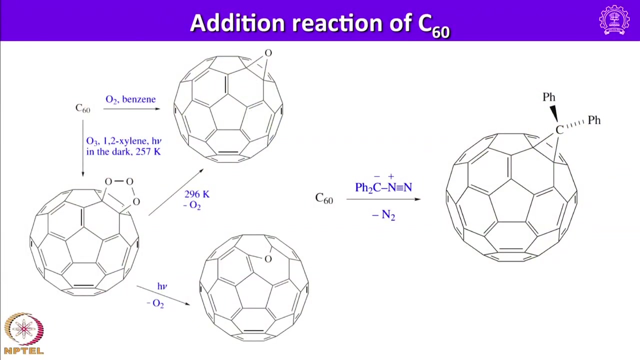 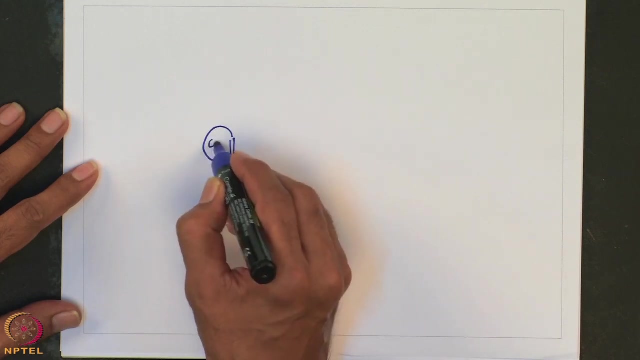 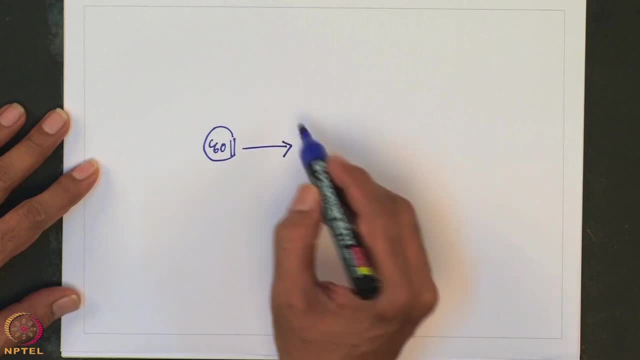 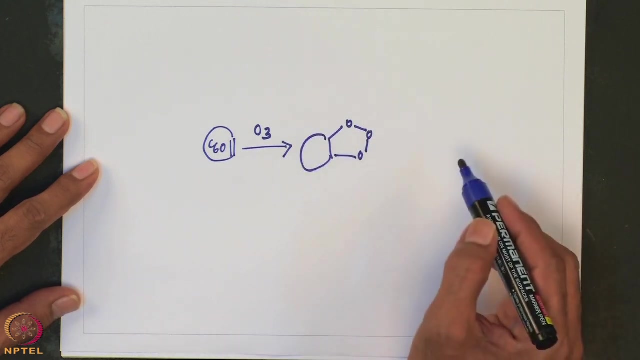 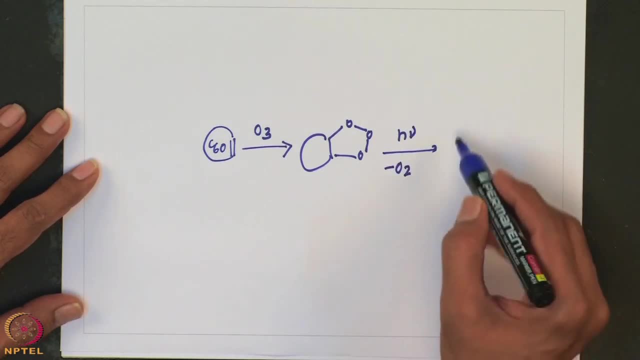 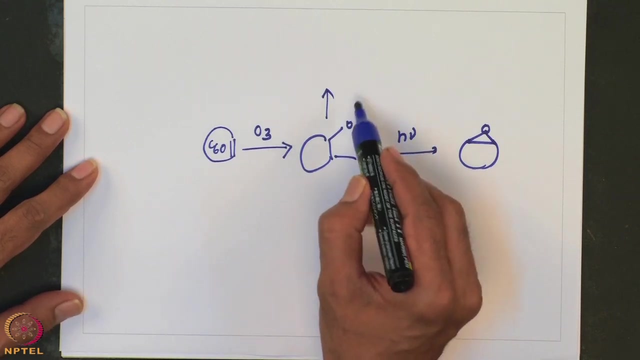 comes out to form oxide epoxide. Or one can take this one and treat with the heated to 296 Kelvin. 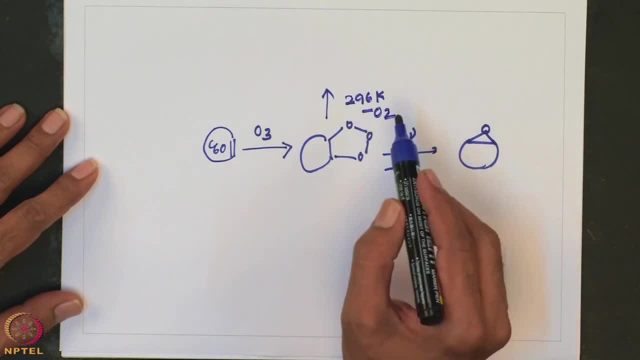 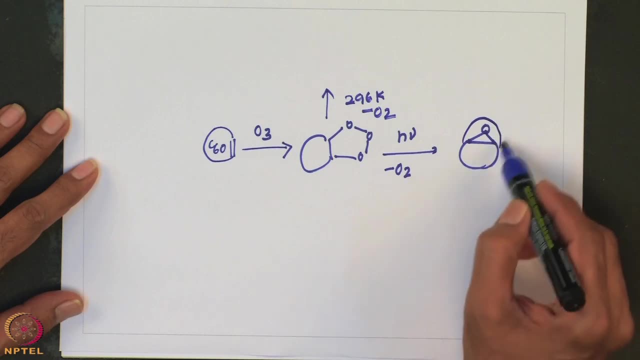 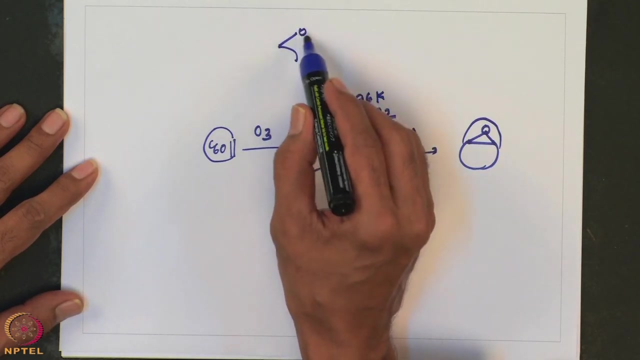 can come out here also and one can also get. Now it will be something like it will be part of it. it will be it opens up one C-C bond it forms, or it can be simply an epoxide. 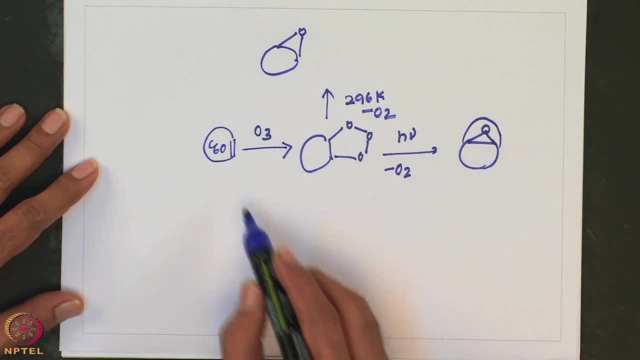 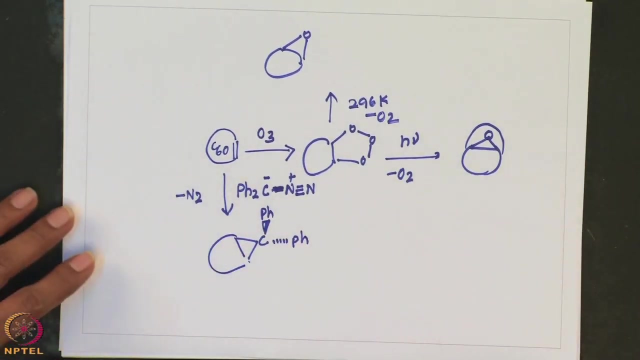 something like this. it can form. And taking C 60 directly, let us say, if we treat this one with this reagent, ok, So N 2 will come out here. So here one can see addition reaction happening here. Ok, So it is diazo compound can be taken and added so that you can carry out several reactions. 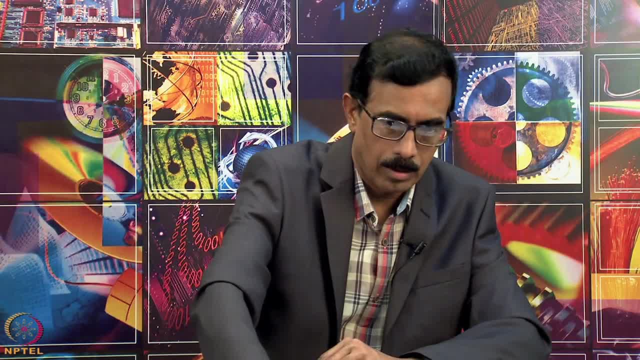 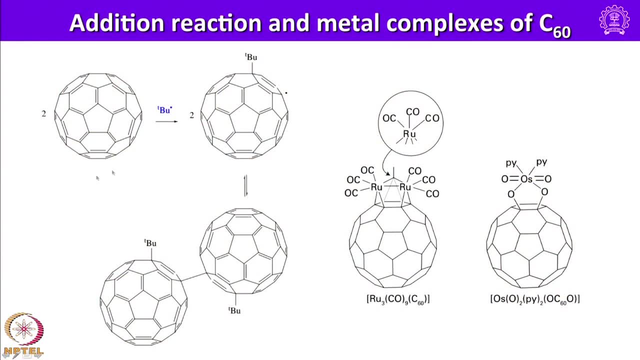 ok, Of course one can also add carbonyls also on to it. You can see here: some of these reactions are shown here. in this one: ok, You can take this radicals and you can add it here. Or you can take Ru CO 3 fragment, ok. Or if you take Ru 3, CO 12, you can do addition reaction. 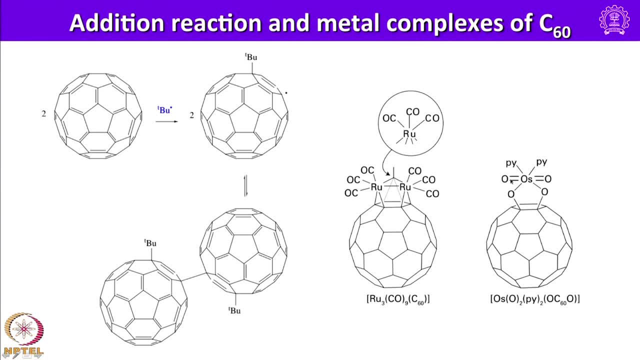 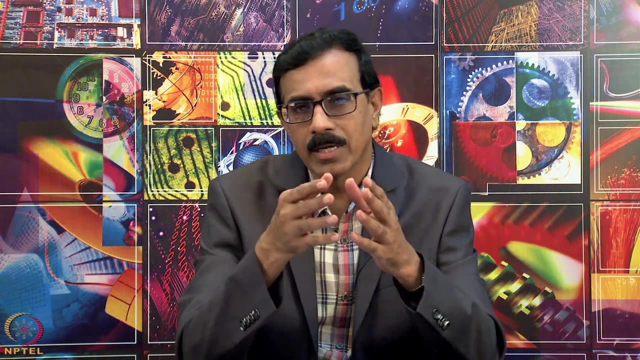 in this fashion, ok, And also one can treat this one with osmium tetroxide in presence of pyridine to form a compound of this type, ok. So these are all. reactions are very similar to reacting some of the species with a single alkene. That means essentially they resemble. the reaction with an alkene. Ok, So let us look into the cationation. Cationation is very, very common for carbon, Then for silicon, germanium and tin. among group 14 elements. The much higher C-C bond enthalpy is compared. with those of silicon, silicon- germanium, germanium and tin. tin means that the formation of compounds containing bonds between carbon atoms is thermodynamically more favorable than analogous compounds. So this is the difference between the two compounds having silicon- silicon- germanium. 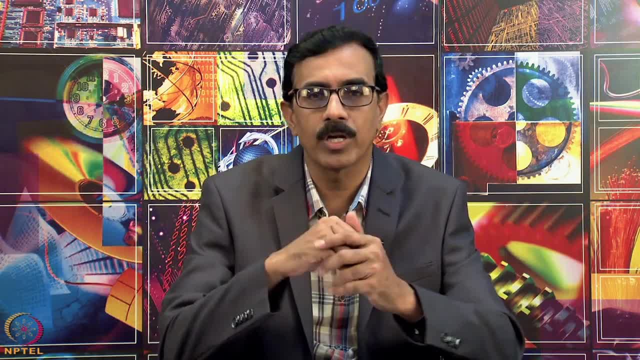 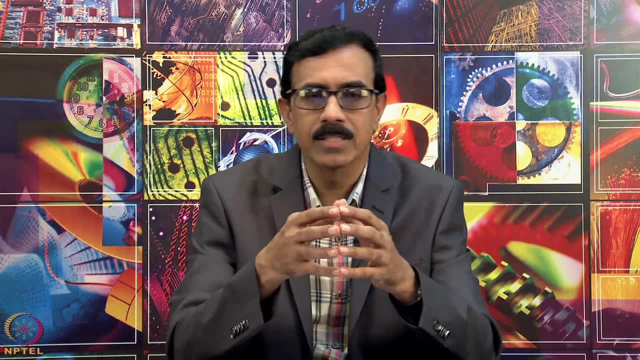 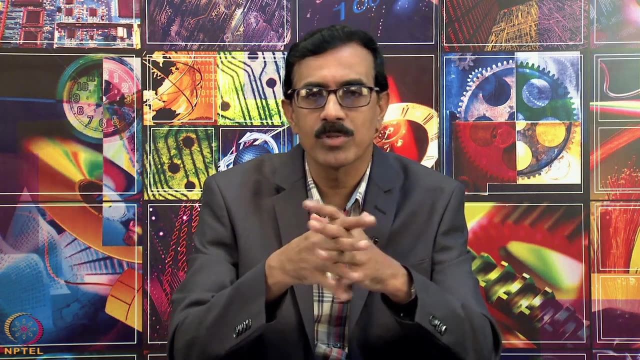 germanium or tin tin bonds On descending group 14, so orbital overlap becomes less efficient as the valence orbital size increases and they become more and more diffuse- ok- as the principle quantum number increases. For this reason, what happens is cationation is. less pronounced among heavier group 14 elements. The backbones of saturated hydrocarbons are composed of C-C bonds. Ok, That is. their formation depends on cationation being favorable. An additional factor that favors the formation of hydrocarbon is the strength of C-H bonds, So stronger than S-I-H. 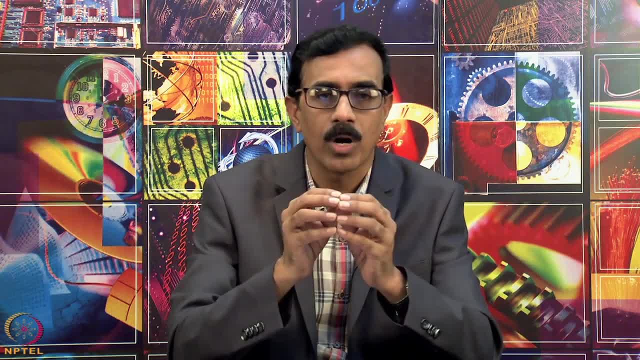 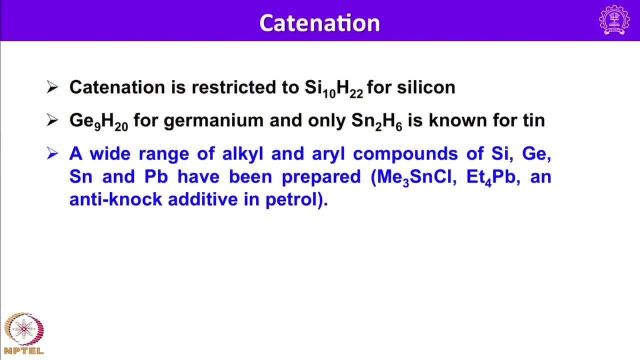 germanium hydrogen or tin-H bonds. Carbon hydrogen bond is much stronger than any of the hydrogen bonds of the group 14 elements. So when we look into the cationation, cationation can lead to all kind of polymers in case of. 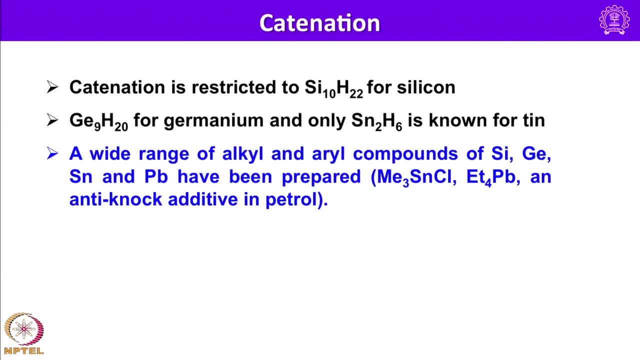 carbon, Whereas in case of silicon it is restricted to having 10 silicon atoms in the chain, For example S-I- 10H22 for silicon, and in case of germanium one can go up to only 9 germanium atoms in a chain: Germanium G-E, 9H20 for germanium, and in case of tin, only dimeric compound is. 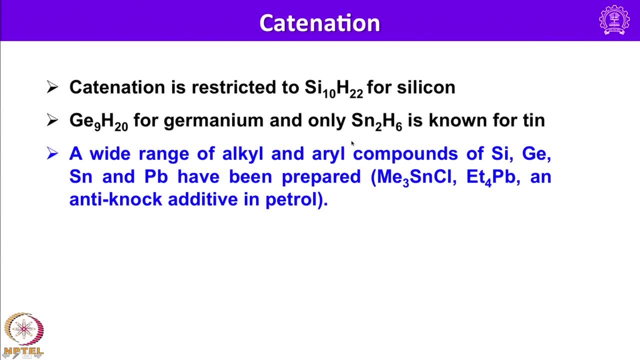 known, very similar to ethane. And of course in case of lead, with great difficulty using very bulky groups one can kinetically control. And of course in case of silicon it is restricted to having 10 silicon atoms in the chain. So in case of silicon it is restricted to having 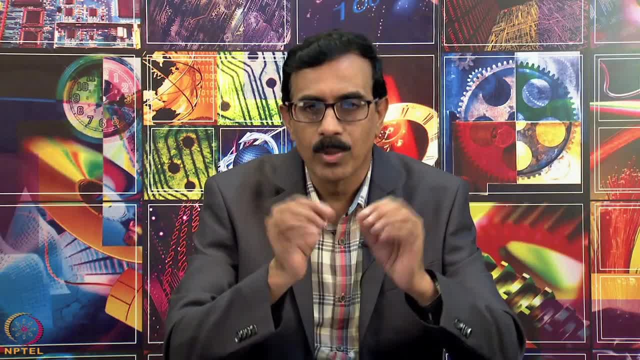 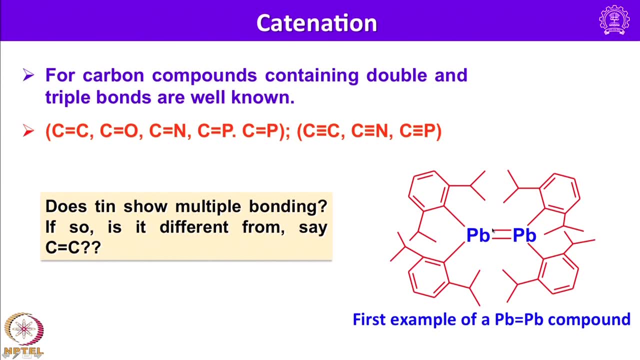 just 10 silicon atoms in a chain. So how we can balance C-I-H bond with nitrogen atom bond. So first we have pureaque form of-cream of or silicon carbon. Let me ask you, how did each of these первex bonds? this- majors areis. 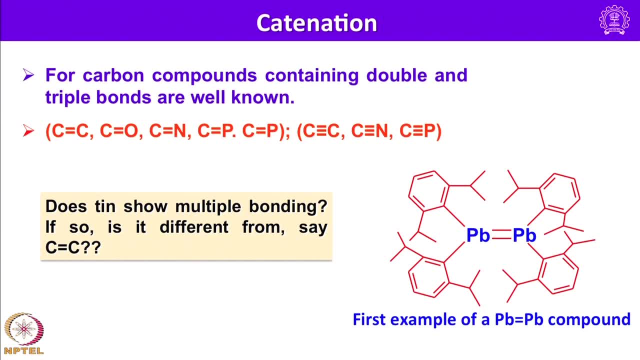 Emilio, chemistry of main group compounds and especially while comparing the bonding of tin compounds with lead and other silicon compounds having more than one bond or multiple multiply bonded main group elements. So this is one example of a dimeric lead compound. Of course you can see. 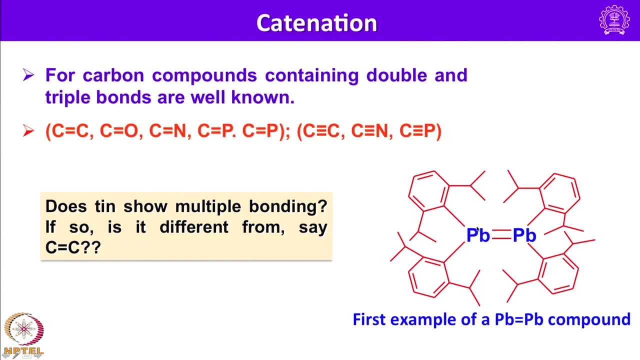 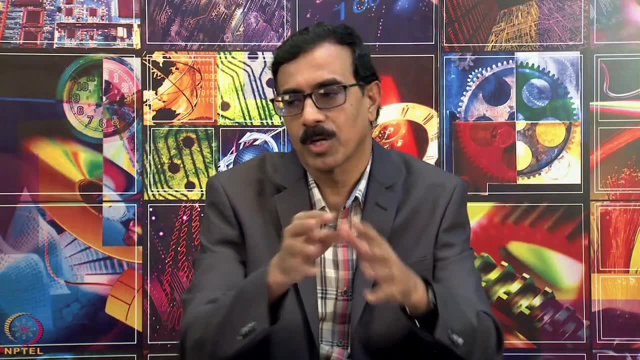 here, this PbPb double bond is stabilized by very bulky groups. We have 2, 6 disopropyl phenyl groups. ok, This is kinetically. this PbPb bond is stabilized. ok, So sulfur 2-catenates. 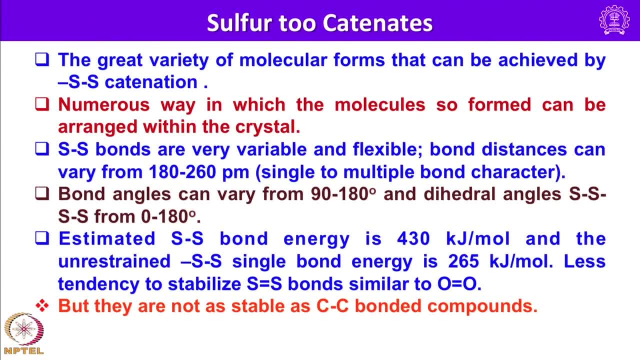 of course, when we look into the catenation, another element in the main group, or among ok the elements in the period table that forms a larger number of catenated compounds, is sulfur. The first one is sulfur, the second one is sulfur. The third one is sulfur. the fourth one is sulfur. 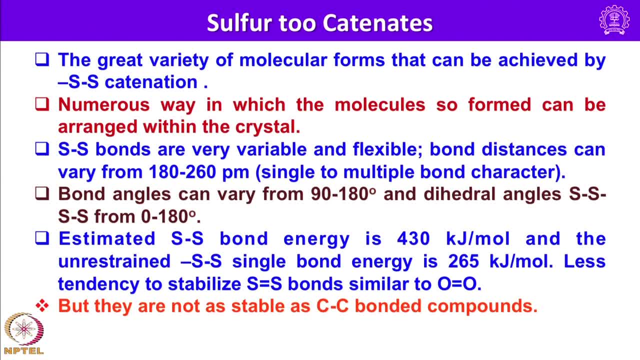 Of course, I will be discussing more about this sulfur chemistry when I start discussion on group 16 elements. Nevertheless, let me compare its catalytic abilities, since we are talking about catenation of carbon. So the great variety of molecular forms can be achieved by sulfur. 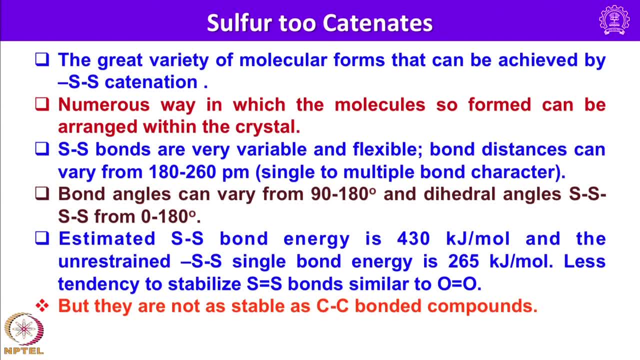 sulfur bond. formation or catenation of Ss. Numerous way in which the molecules so formed can be arranged within the crystal. Ss bonds are very, very variable and flexible. Bond distances can vary from 180 to 260 picometer. Some, there is some. 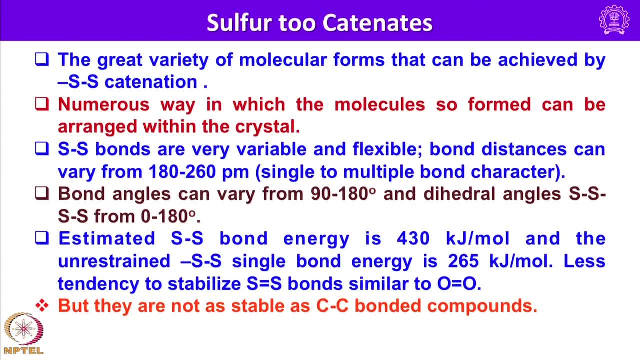 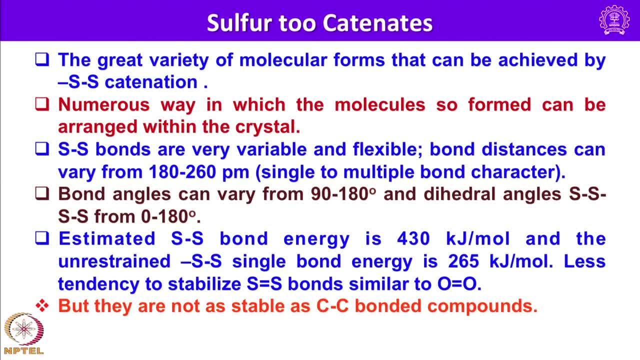 kilojoules per mole and the Ss bond energy is 430 kilojoules per mole. The unrestrained Ss single bond energy is 265 kilojoules per mole, So less tendency to stabilize Ss bond similar to OO bond. 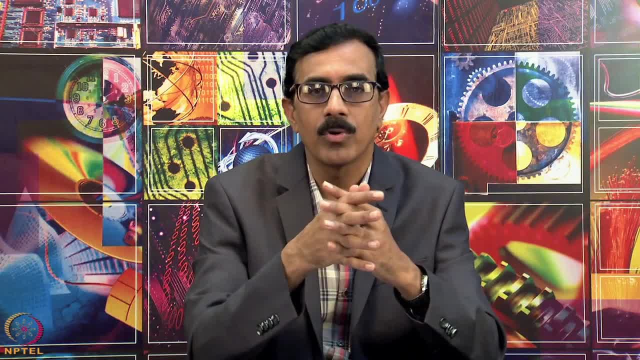 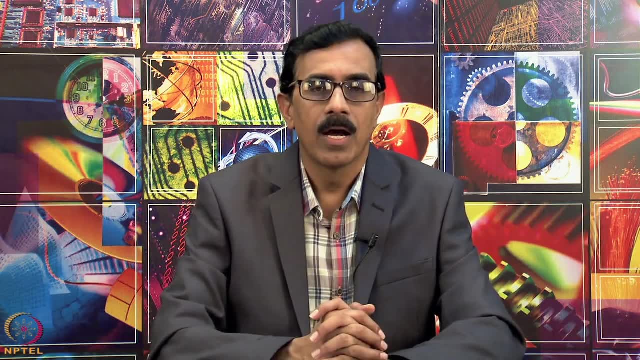 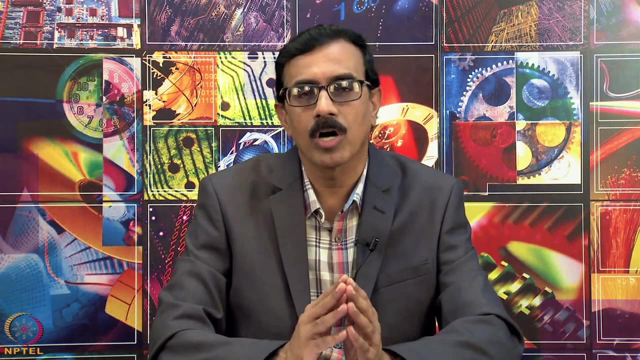 and, but they are not as stable as carbon carbon bonded compound. nevertheless, it shows moderately stable catenated compounds. So catenated halides are another important class of compounds similar to extensive range of hydrocarbons. Diverse range of halocarbons are known, especially chloro compounds. 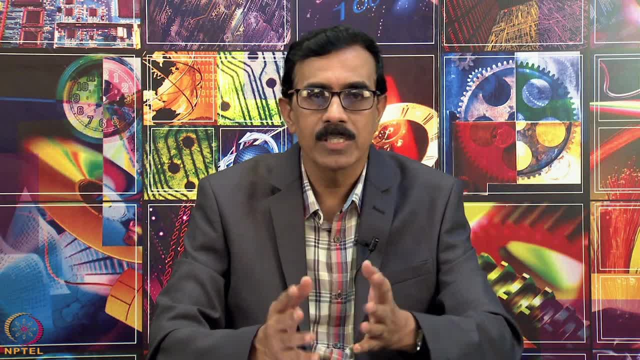 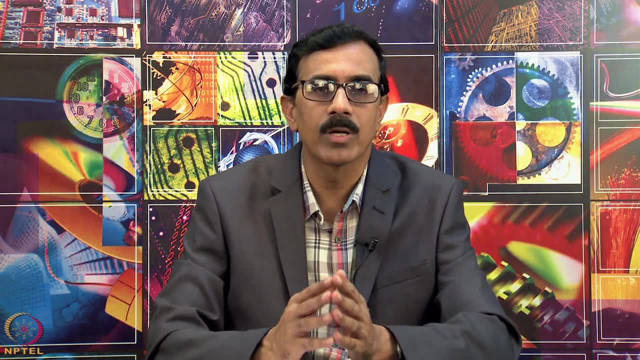 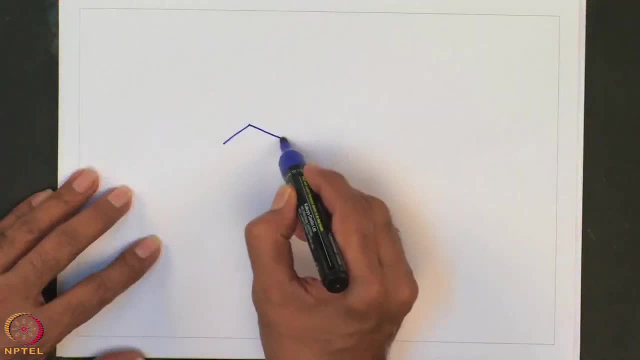 fluoro compounds as well as fluoro chloro compounds together, Best example being poly tetra fluoro ethane, and that is also called PTFE, an extremely stable polymer finding numerous applications, and this PTFE has something like this: the structure ok. 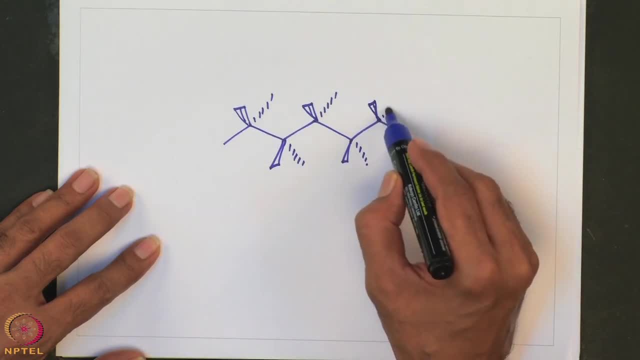 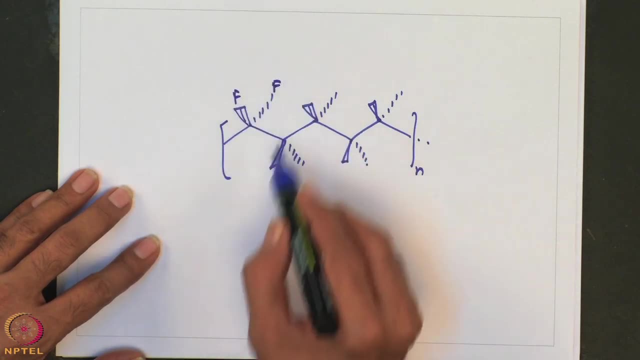 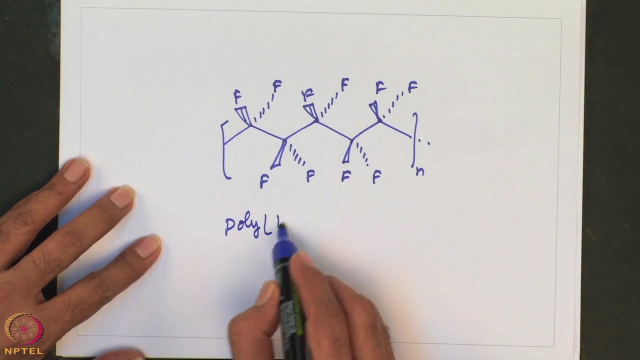 It goes, and all are fluorine atoms. This is called poly tetra fluoro ethane. So this is the structure of poly tetra fluoro ethane. So this is the structure of poly tetra fluoro ethane. So PTFE for silicon. a large number of higher halides are known containing chains of silicon. 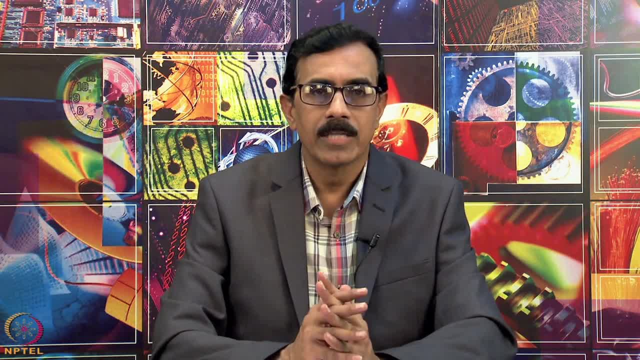 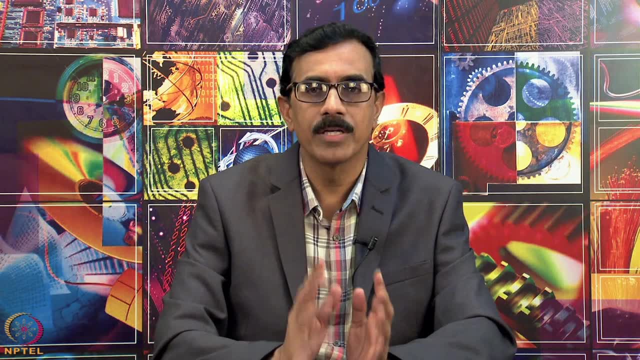 atoms analogous to the polysilanes, Germanium, tin and lead form. few analogous of the silicon compounds because of the lowest stability of EE bonds going down the group and the increased stability of the diethylene bonds. So this is the structure of poly tetra fluoro ethane. So this is the structure of poly tetra fluoro ethane. So this 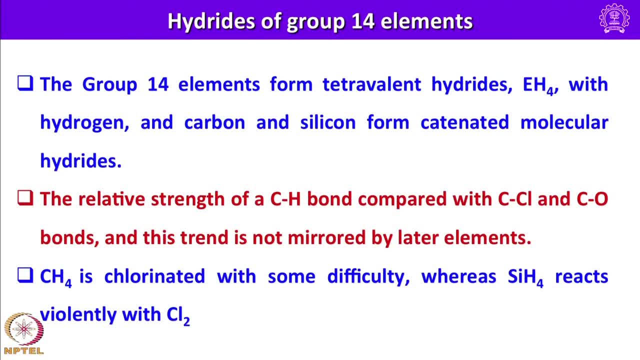 PTFE for silicon is an important element. now we now talk about poly ،- this is a term term- various parameters, and it is called poly células and they are very much related to the cell casing, the cell spaces and to the differences of the vivobook in a circuit. 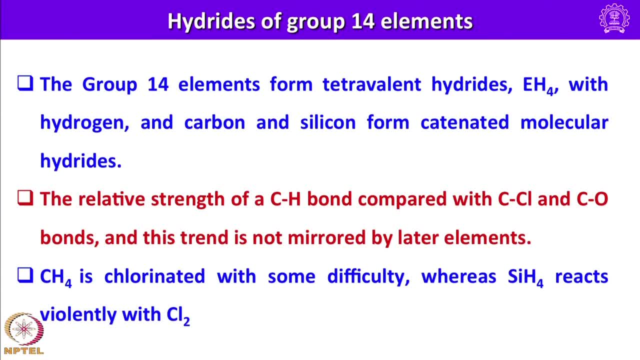 these are signal medium to the liquid and are usually used for the waiters and or culinary activities. aga violent halorides. let us look into the hydrates of group 14. elements There group in the chain and each one is having 2 hydrogen atoms. ok, The relative strength of a CH bond. 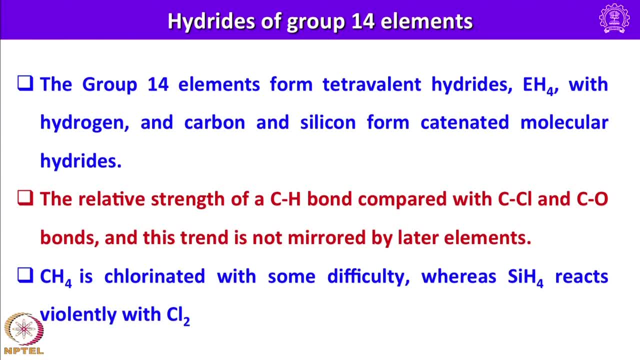 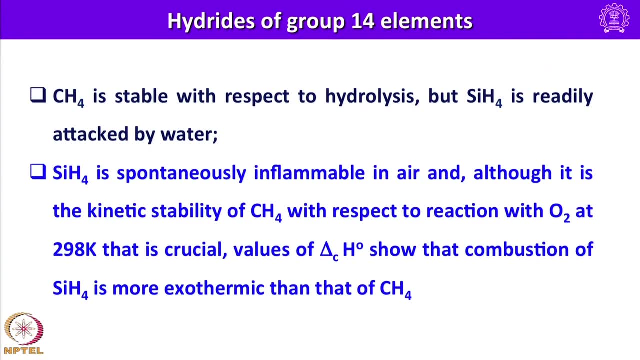 compared to CCL and CO bond, and this trend is not mirrored by later elements. CH4 is chlorinated with some difficulty, whereas SiH4 reacts violently with chlorine. ok, CH4 is very stable with respect to hydrolysis, But a SiH4 is readily attacked by water. Here the reactivity of SIH4 is are purely 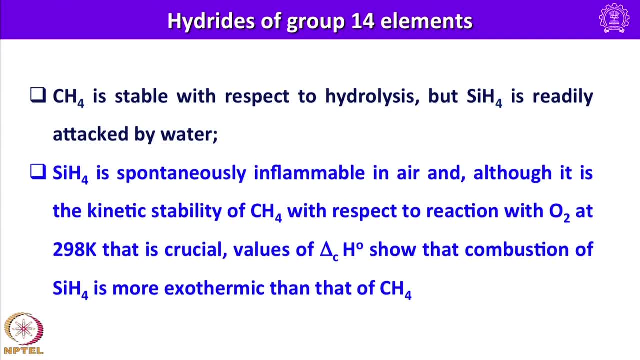 kinetic SiH4 is spontaneously inflammable in air and although it is the kinetic stability of CH4 with respect to reaction with oxygen at 298 Kelvin there is crucial. The values delta CH naught shows that the combustion of SiH4 is more exothermic than the chamber temperature, So water is applied. 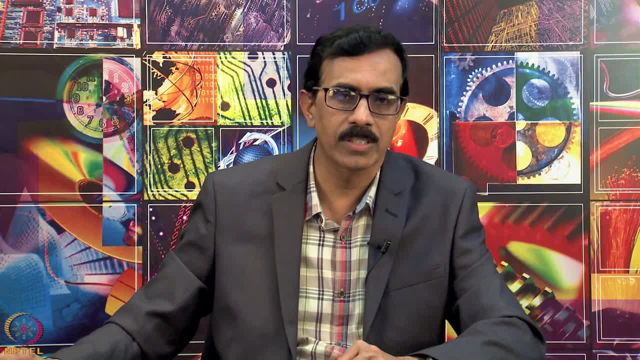 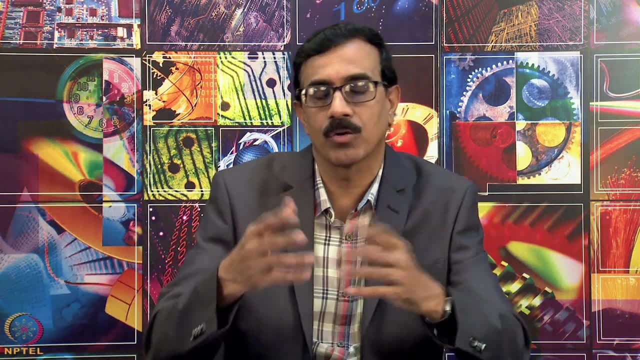 to the hot water. two sự fuera reattτι Blendty. see, there is concentration of CO state of this, that of CH4, as I said, it is one is exothermic, another one is kinetic. ok, I will. I shall explain later when I talk about the reactivity of SiCl4 with respect to CCl4.. CCl4 is not prone to. 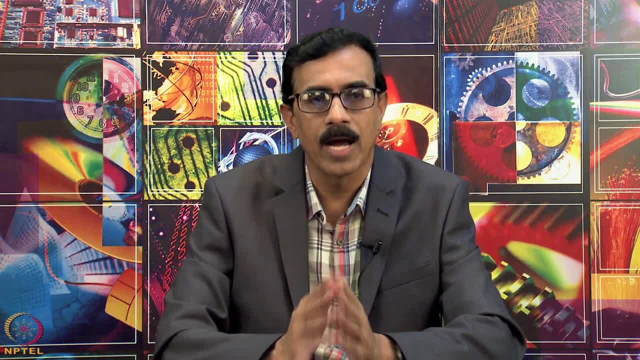 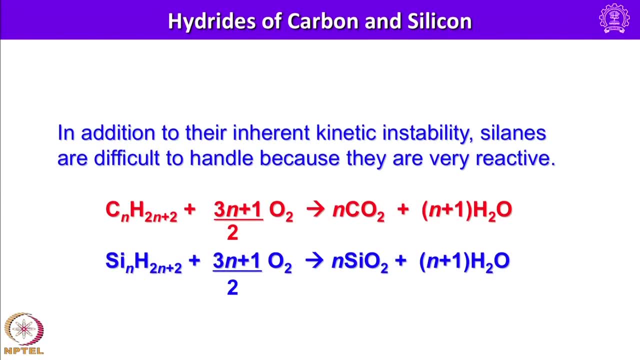 hydrolysis, whereas SiCl4 can undergo readily hydrolysis. ok, So, in addition to their inherent kinetic instability, silanes are difficult to handle because they are very reactive. For example, if you take here, this is a typical reaction of a carbon hydride or hydrocarbon reacting with 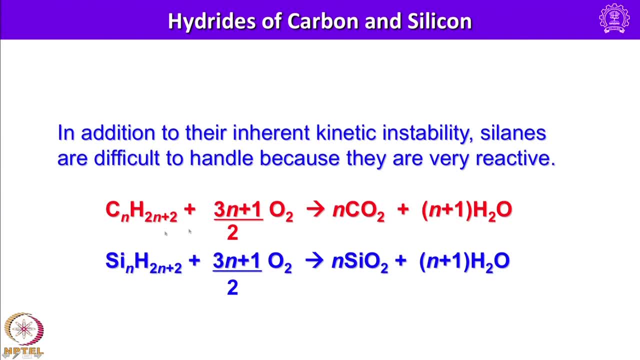 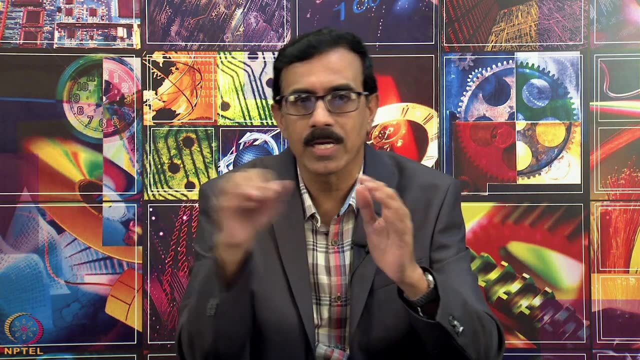 oxygen to give water and carbon dioxide. Similarly, if we compare the reaction of silane with oxygen, it gives silica, that is, SiO2 plus water. So in fact, both the reactions are thermodynamically favored to proceed together Towards the right. ok, the major differences not apparent in the stoichiometric reaction is the: